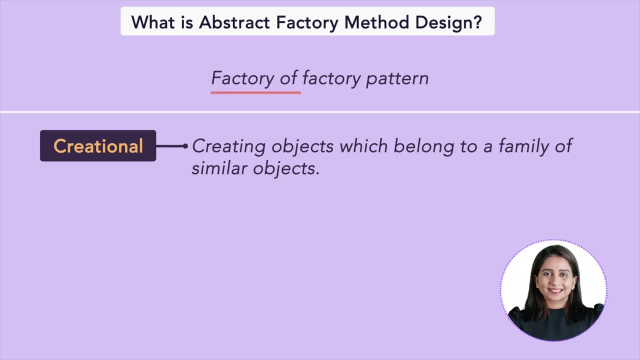 which are of similar type. here we are using a factory of factory to create a factory of factory Create objects which belong to a family of similar objects. We can understand more when we go into the examples. Just like factory method design pattern, this pattern is also implemented using 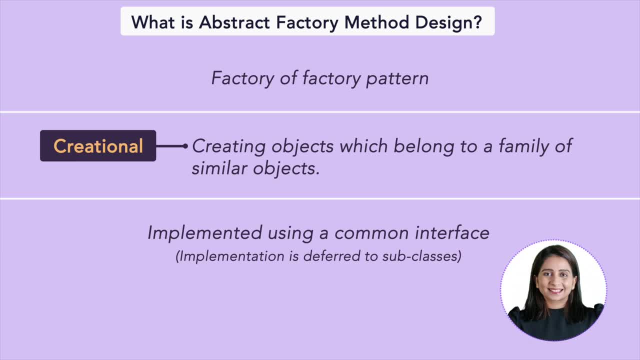 a common interface and the implementation is deferred to the subclasses, or the concrete classes as we call it. One example of abstract factory method design pattern is java document builder. You can check that source code and if you want to know more about the java document builder, 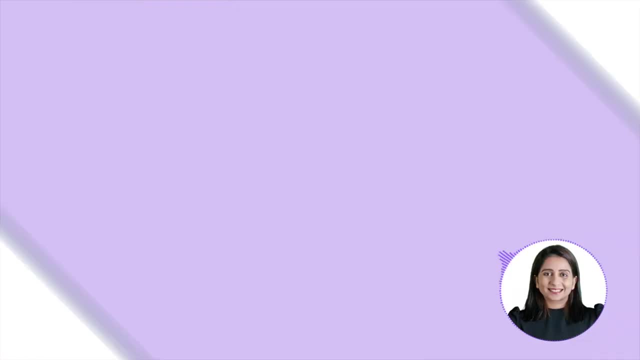 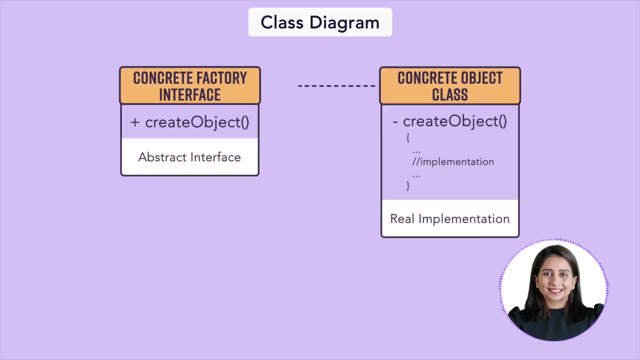 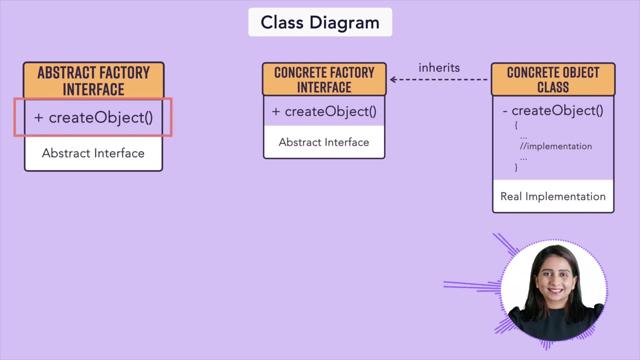 understand more about how this pattern is implemented. If we talk about the class diagram of abstract factory method design pattern, it's very similar to the factory method design pattern, except that there is one more extra interface on the top where you have your function which allows you to create objects which internally uses concrete factory and the exact implementation. 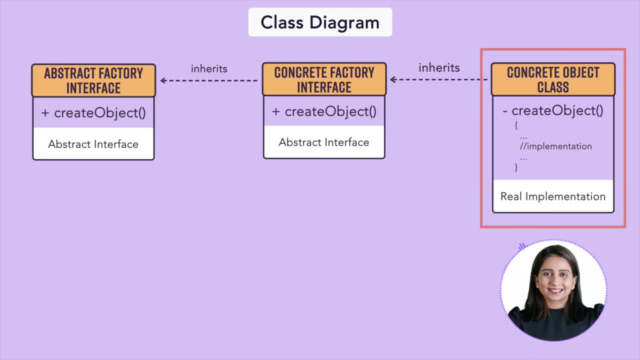 or the instantiation of the objects lie in the concrete object classes. There is some logic in the concrete factory implementation as well, where it is decided which factory will be utilized to create this concrete object and then how that object is created will be decided in the implementation of the concrete object. Let's understand how the code flow will look like. 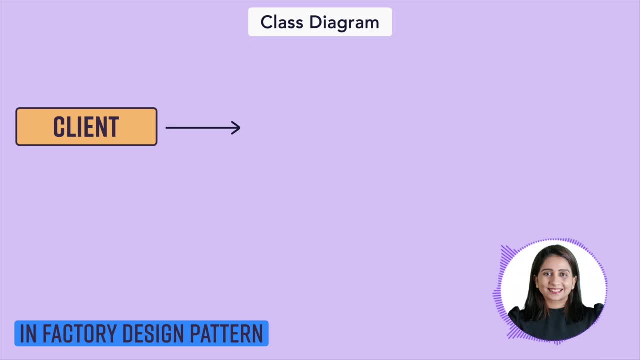 In case of factory pattern, we used to have a client which used to call a factory and on the basis of some parameters, that factory will call the functions which create concrete objects. In case of abstract factory, the client is going to call abstract factory on the basis of some parameters, that abstract factory. 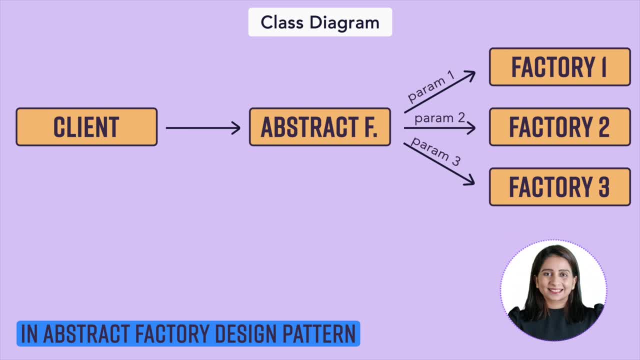 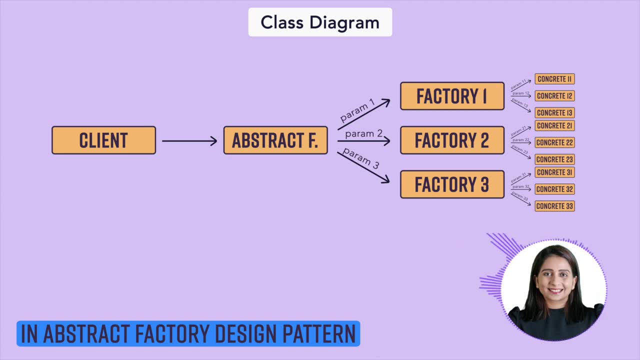 will call the implementation of one of the factories which internally will call the implementation of their respective objects and return that object. So it is just one more additional layer of abstract factory over here which decides which factory to call and then that factory decides which concrete implementation to call, As usual. 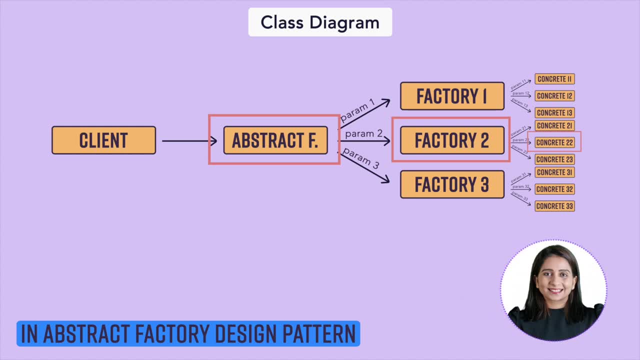 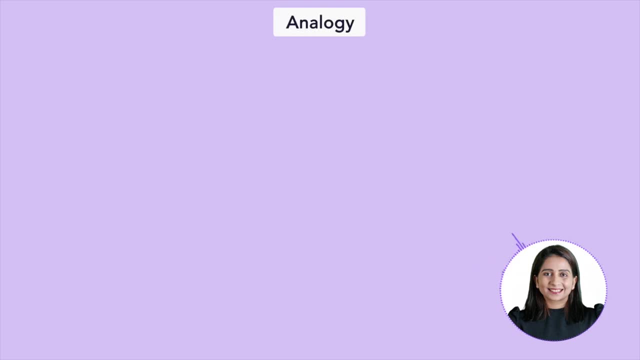 we cannot complete any of our video without an analogy. So let's understand the abstract factory method pattern using an analogy, Just like in the previous example, we discussed the example of a factory which produces lids and, on the basis of different type of lids, different sections of factory. 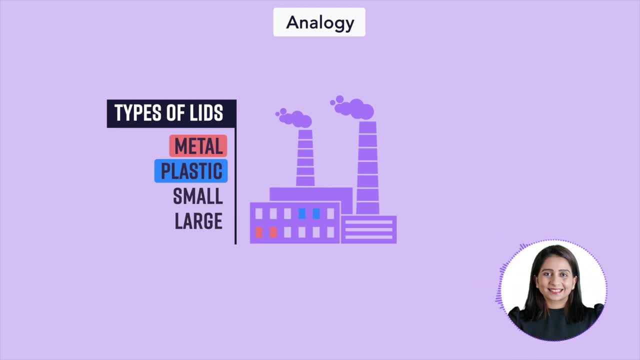 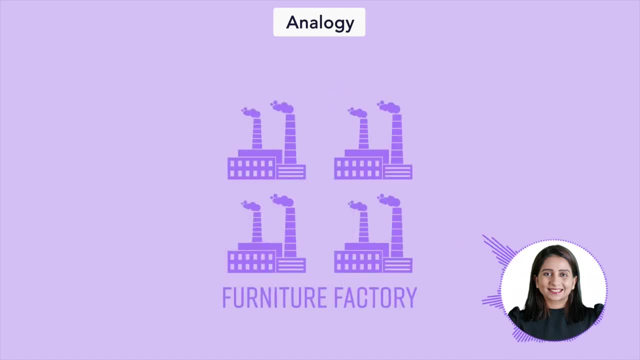 produce those lids, but the client has no idea how those lids are produced. Similarly, now, this time, let's say that there is a huge furniture factory which is a collection of some smaller factories. So the client is going to place order for chair or sofa or table. 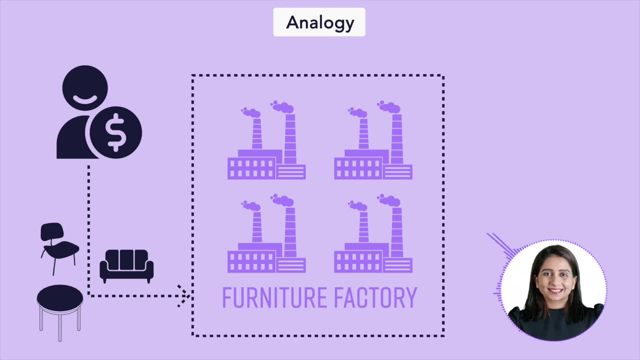 Ultimately, this abstract factory will give a common interface such as, like, you can place order for a piece of furniture, which can be chair, sofa or table. Internally, depending on what order has been placed, whether it's a chair or a sofa or a table, this factory will send that order to. 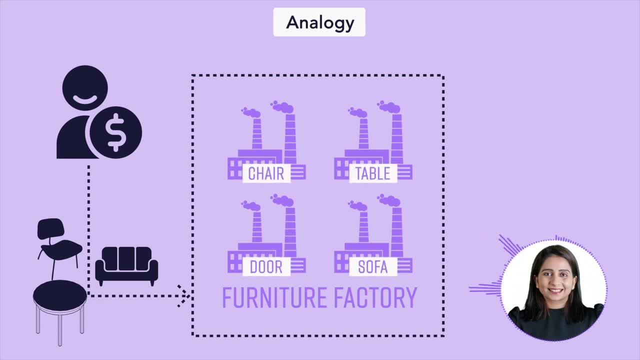 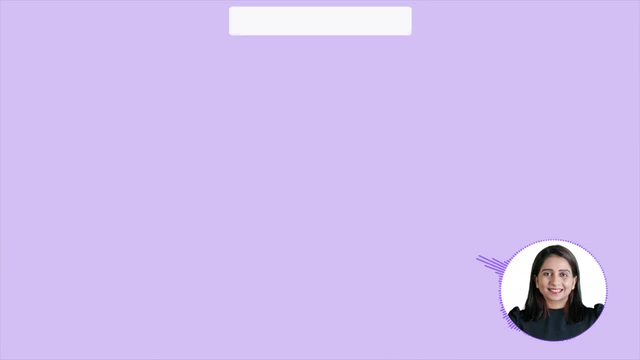 its respective specialized factories for that furniture to be manufactured and then returned to the client. So this is a factory of factories. Now let's understand from an implementation perspective how you are going to implement your own abstract factory method design pattern. Let's say that you want to go to a college. For that you have written an exam and you have a. 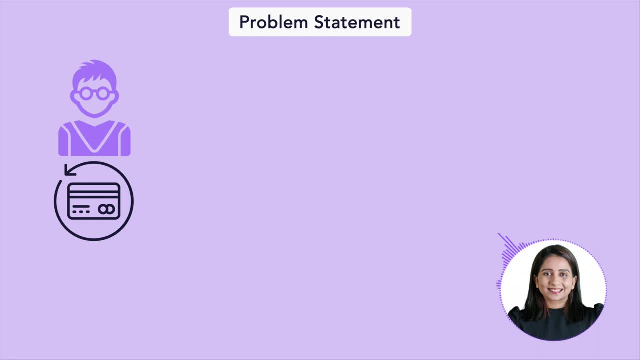 score. On the basis of the score of your exam, you are going to get an admission into a college and you need an admit card for that. Now there can be different admit cards for different universities and you can get admitted to different universities on the basis of your score Also. 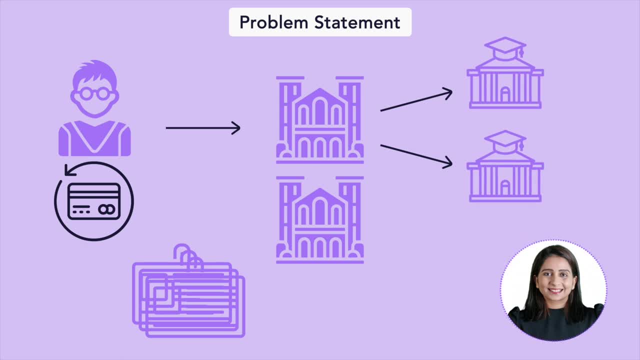 every university will have different type of colleges And every college will have a different type of fees. So our task here is to write code so that we can get a different kind of admit card on the basis of the score that we have received in the exam and also on the basis of the choice of subject. Let's understand. 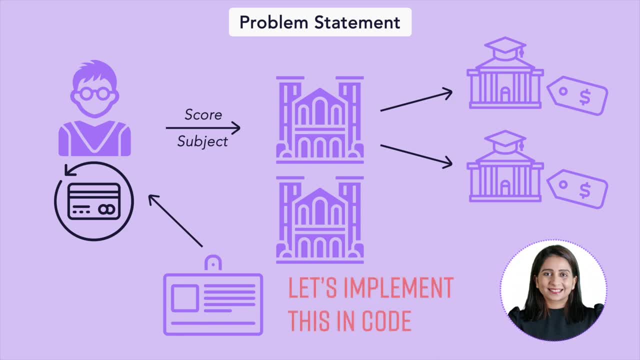 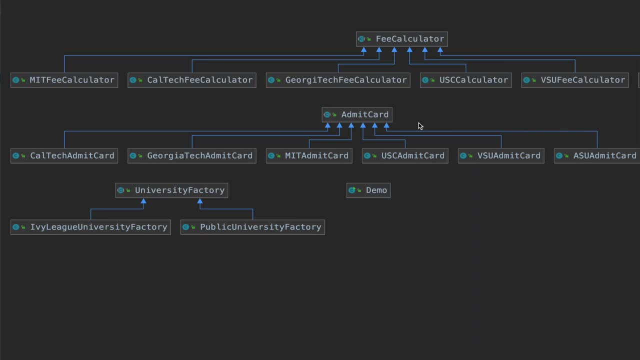 the implementation of abstract factory method pattern using this code example. In this example, we are going to create different admit cards on the basis of the exam score and the type of course student wants to choose. In this example, we have a demo class over here which is going to be the. 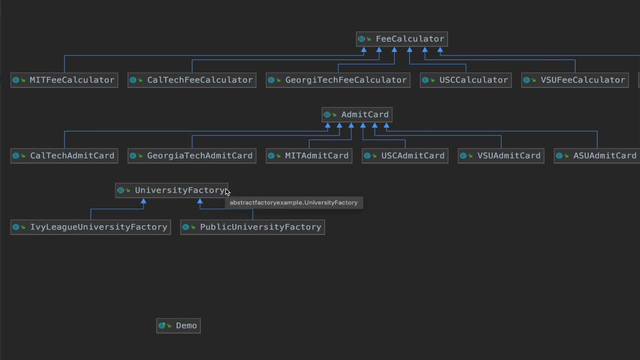 client of these factory classes. It is going to call university factory, abstract university factory, which will return either this particular factory or this factory, depending on the score, And then, using this factory, we will try to instantiate an admit card. Similarly, on the basis of this factory, we will also try to instantiate or get a fee calculator. 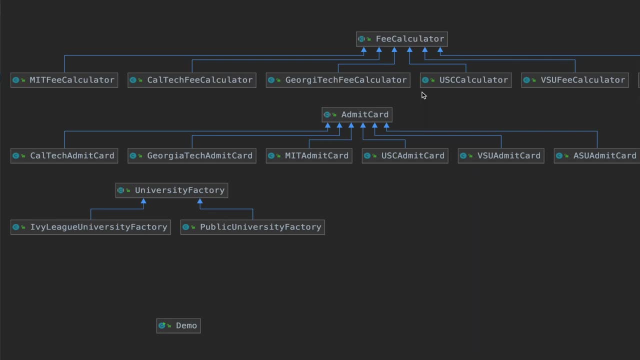 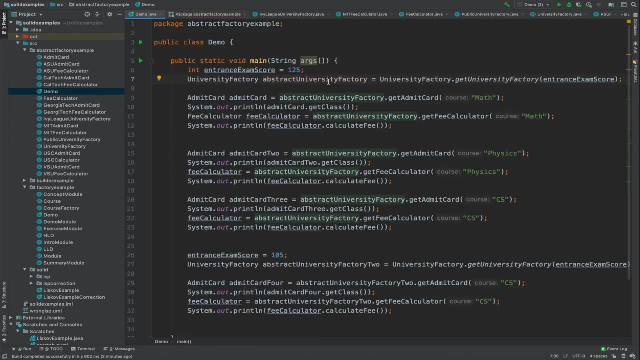 for a particular university that the student is going to be admitted in on the basis of the course and the score that they have received. Now Let's try to tackle this from the client class. In the client class, as you can see that I have initialized an. 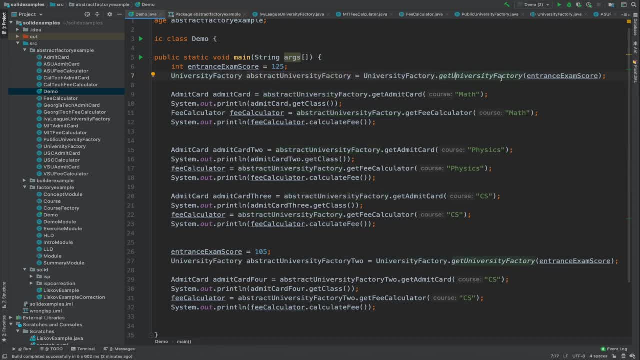 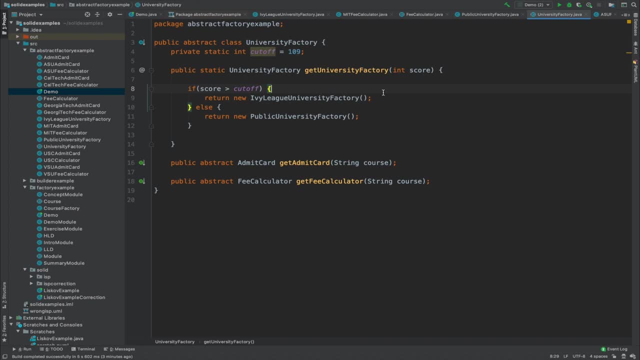 abstract university factory which is calling get university factory. The subtopic parameter is applied for entrance exam score. If you try to get into the definition of this function, how it is finding out which factory to return, It is checking the score and the cut off. If the score is greater than cutoff, it is returning Ivy lea university factory. If the 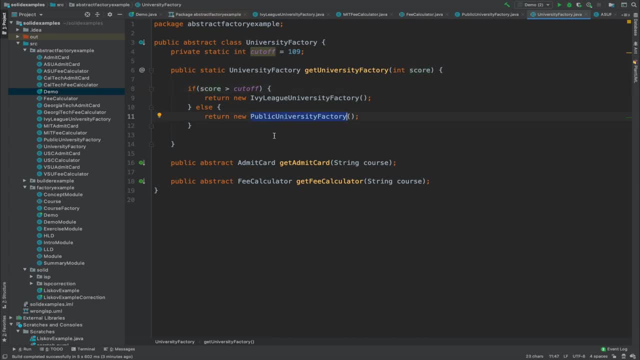 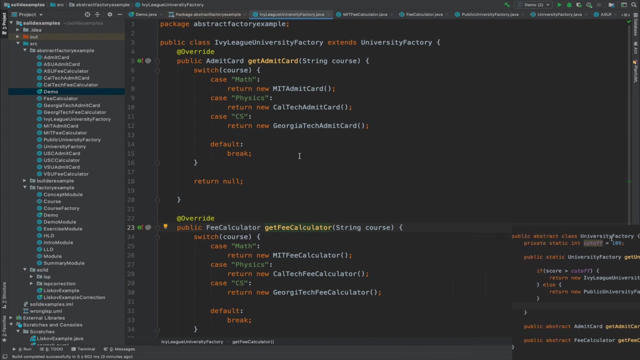 is less than cut off. it is returning public university factory. Now you can also see that every university factory have two more abstract methods, which is get admit card and get fee calculator. That means that both these factory classes have to implement these functions: get admit card and get fee calculator. The response to these functions is calculated on the basis of. 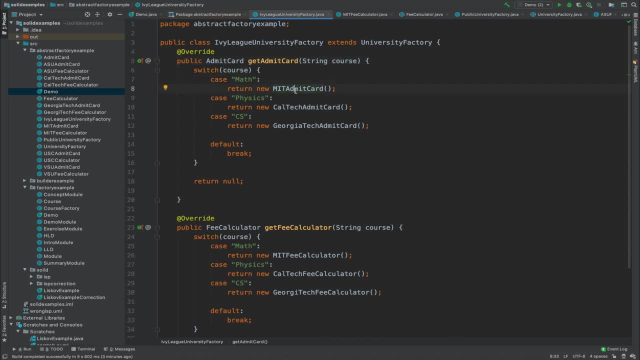 the course. On the basis of the course, an admit card with respect to a particular college is written. If it's a math course, MIT admit card is written. If it's a physics course, Celtic admit card is written. If it's a CS course, Georgia Tech admit card is written. The same logic gets. 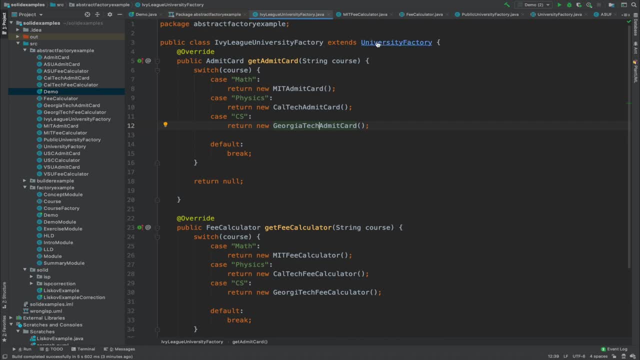 applicated in getting the fee calculator as well. If we go back to university factory where we have public university factory as one of the factories that is written, it also follows the same methods and the same logic, just like the Ivy League university factory, with the exception of: 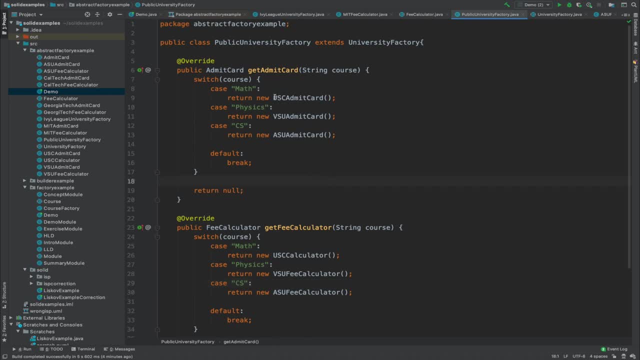 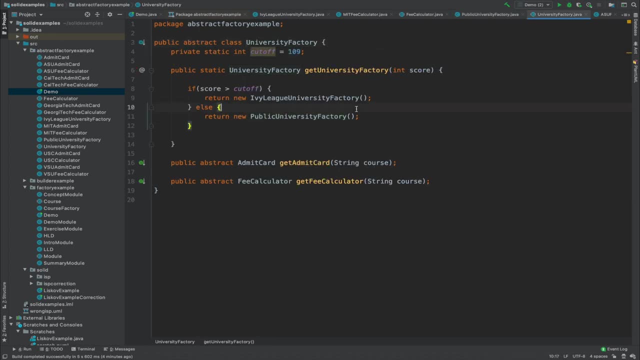 different colleges and different fee calculators. So, as you can see, the same logic is used in getting the fee calculator. If we go back to university factory, these particular classes are going to have the exact implementation, whereas the university factory class is going to decide which factory is returned to the client code. If you come back to 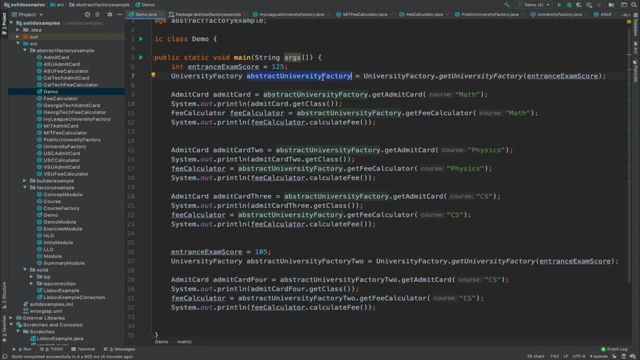 the client code, you realize that this abstract university factory gets the particular factory on the basis of entrance exam score and then this particular client class or the demo class has no idea how those factories are getting returned from this function and also how this admit card and get. 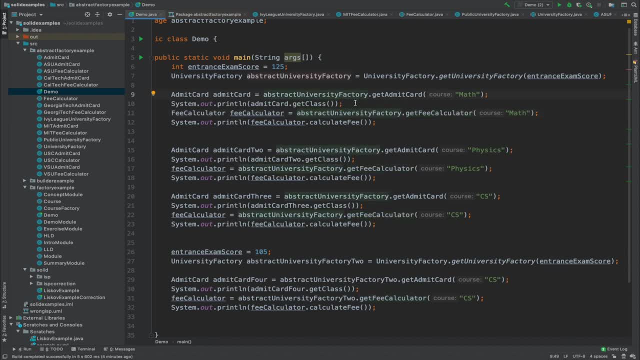 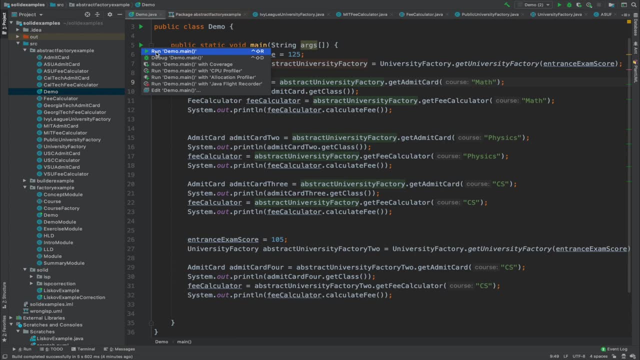 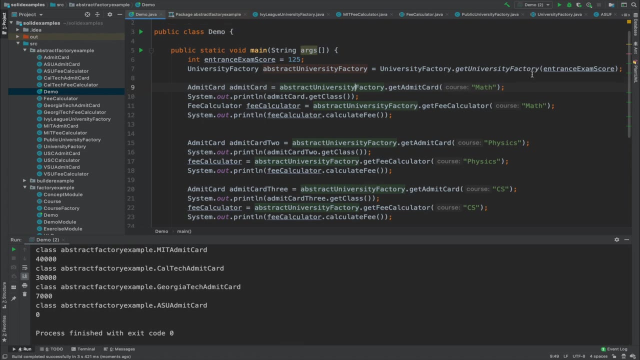 the fee calculator is getting written from this university factory instance, But we, being developers, can actually check what is going on in under the hood. So let's run this code and try to understand what response we getwall release. As you can see, in the first case where the score was 125 and the course was MAC, we got the admit. 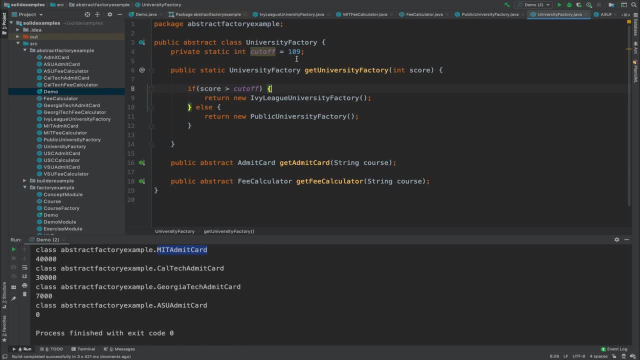 card for MIT. If we go back to our code, we can actually verify this. the score was 125, which is greater than the cut-off «$5». So I took this load and this test and the customers is fineをük addicted to it, but they are. 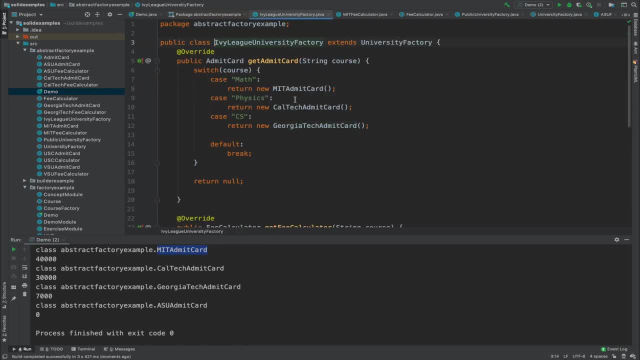 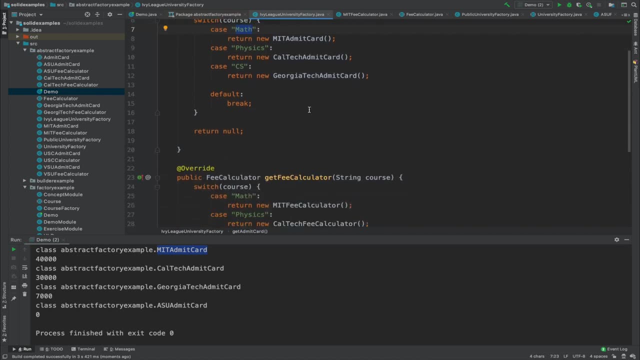 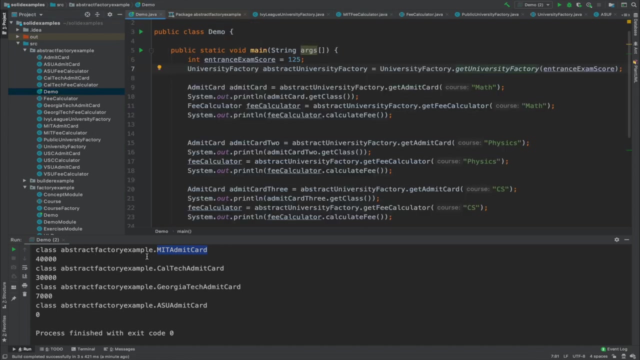 was 125, which is greater than the cutoff score, which will give us an ivy league university factory. and since the course was was math, it will return us the mid admin card. let's also check what is the fees for mid admin card. the fees is 40 000.. if we come back to our response, you can see that. 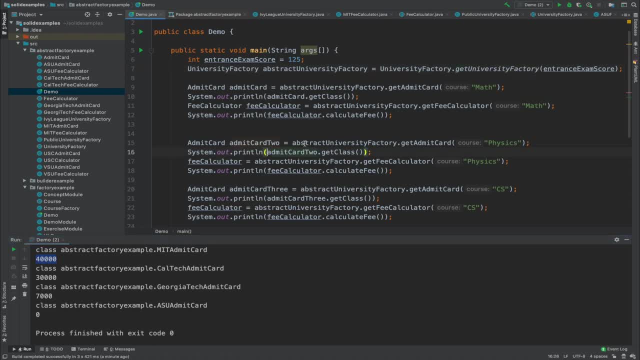 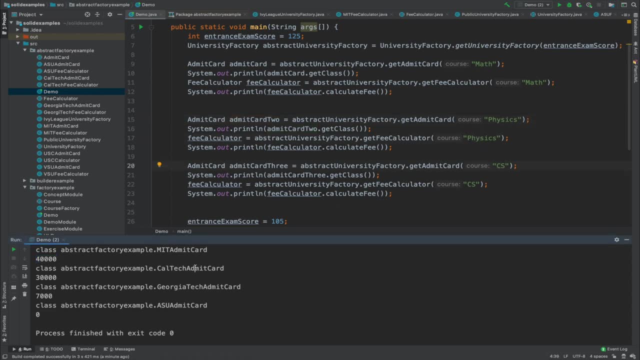 we have mid admin card here and the fees is 40 000.. the same thing is demonstrated here, with the same score, but different courses like physics and cs, and you can see that you got different admit cards, like caltech and georgia tech and with their respective fees. some of you might know. 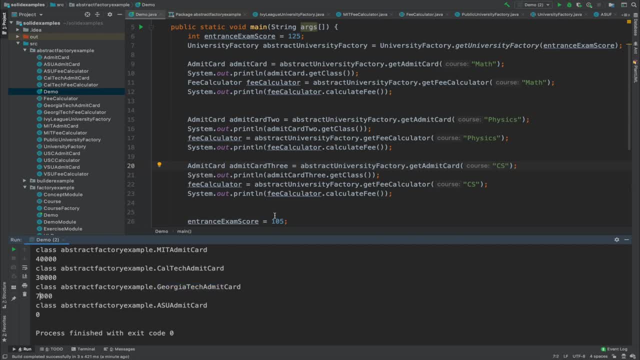 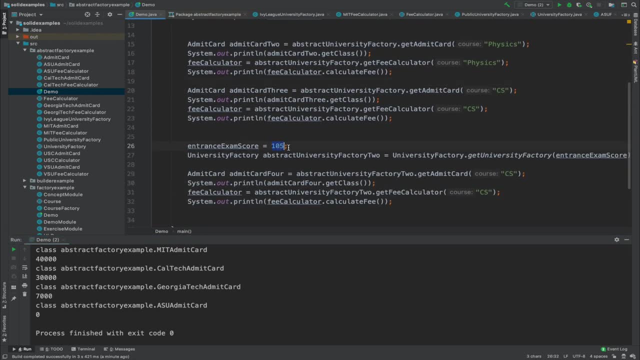 what i did here with respect to georgia tech and the 7000. if you don't know, check out the other videos and you will find out the secret behind this. now, what happens if we change the score? if we change the score to 105? what happens then? if we do that, then, as you know, we are going to get 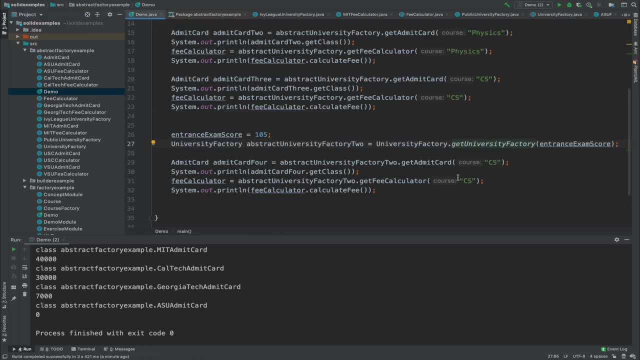 public university factory and on the basis of this particular course, cs, we are going to get different fee. so here we got a su admit card and the fee is zero here. so, as you can see that we can instantiate different type of admit cards from an abstract factory which internally has two more factories and using 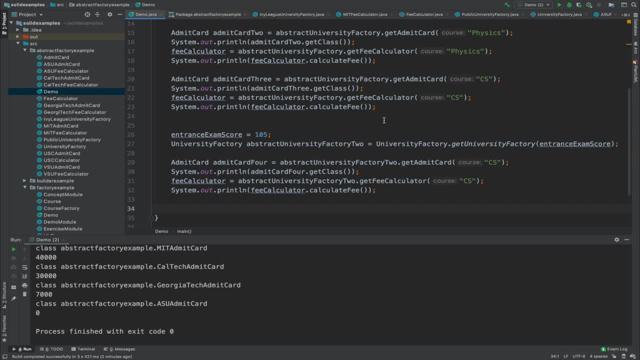 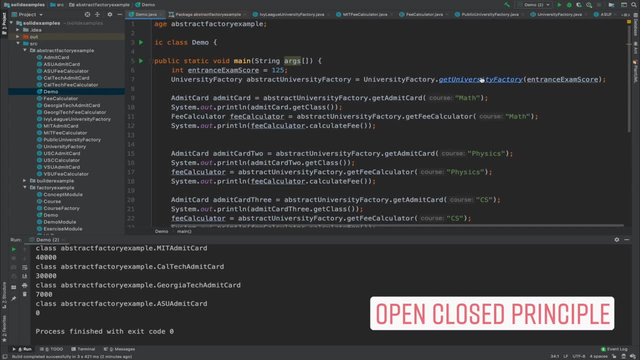 those two more factories. there can be different type of objects that can be instantiated and their implementation can be completely different. how this code base supports open, close principle. if we go back to this, get university factory class. you can add here as many conditions as you like and 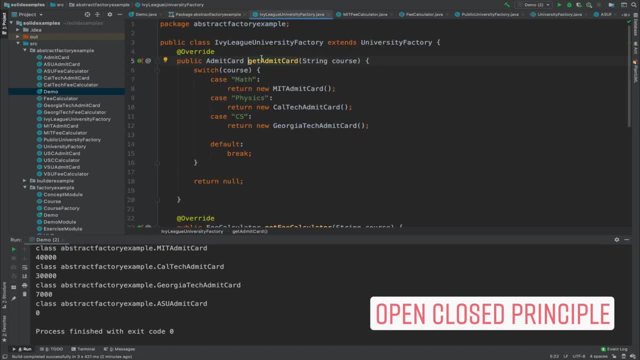 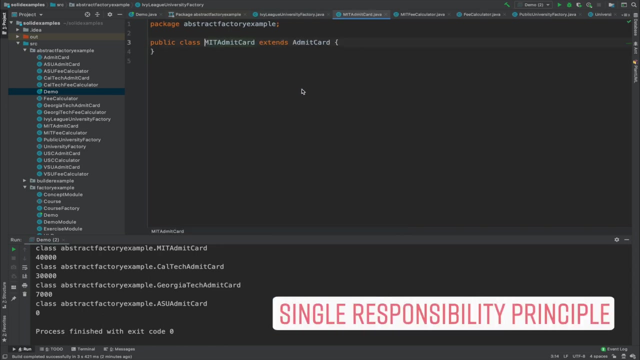 similarly, if we go to the implementations of this particular ivy league university factory- or public university factory for that matter- you can simply add more switch cases here and different kind of admit cards. that way these classes are open for extension, but if you go to just mit admit card, 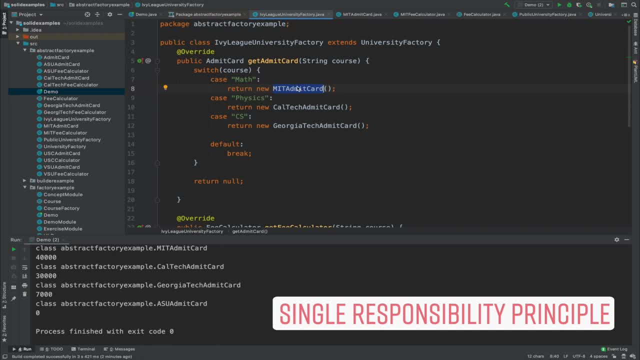 you can see that this particular implementation is specific to mit admit card. so if you want to change implementation of mit admit card, you don't have to touch caltech admit card or georgia tech admit card. that way these classes are closed for modification or changes in. other classes won't.